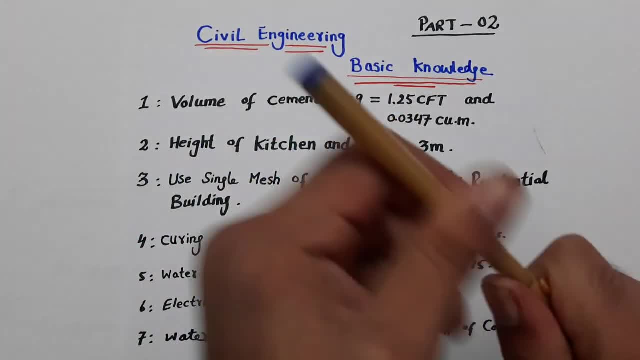 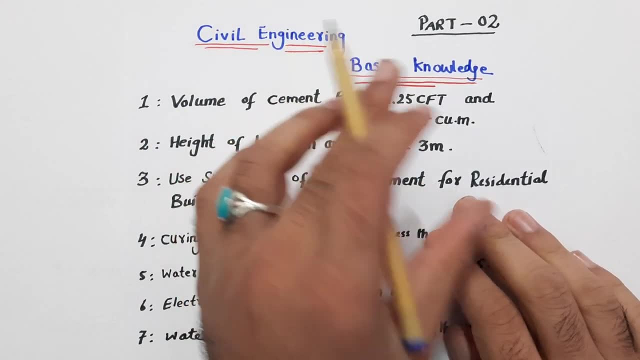 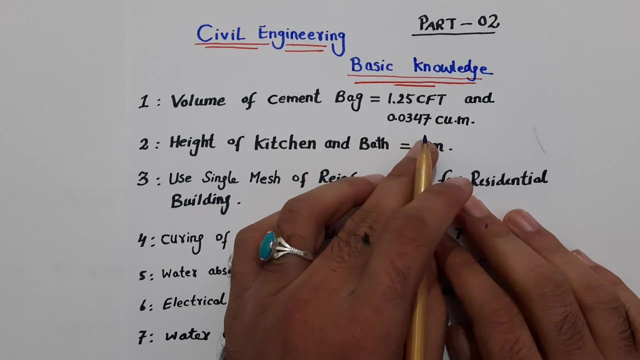 Assalamualaikum, beautiful people. guys, this is part second: civil engineering: basic knowledge. before this video, i discussed part first, if you need part first, so the link is in the description of this video, so watch the part first also, because that one is also very important. so, guys, 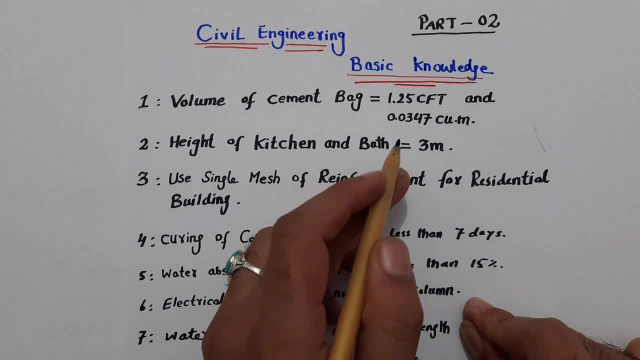 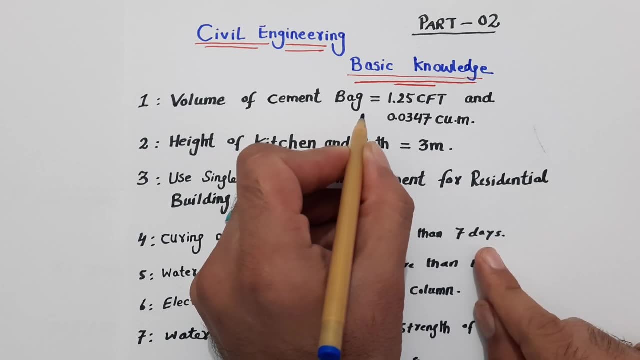 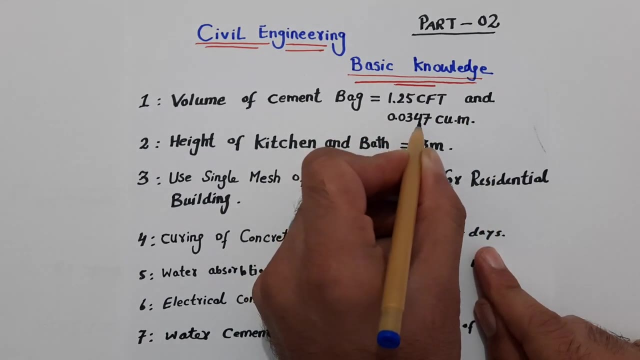 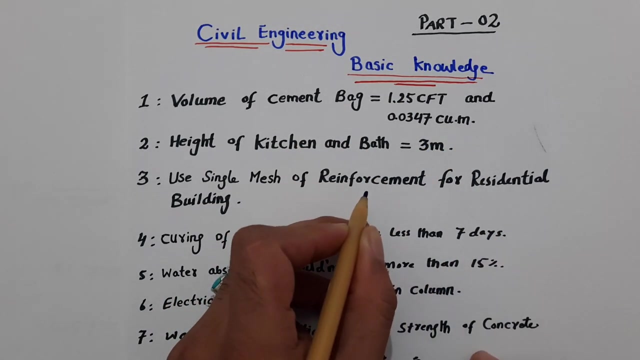 in civil engineering basic knowledge, part two. we have the first one, volume of cement bag. what is the volume of cement bake? the volume of cement bake is 1.25 safety and 0.347 cubic meter. okay, this is the volume of cement. the second one is height of the kitchen and bath should be. 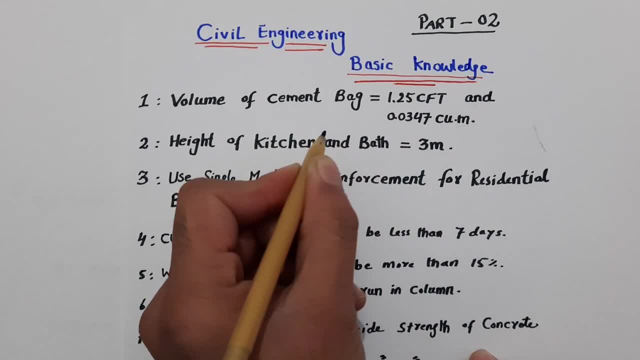 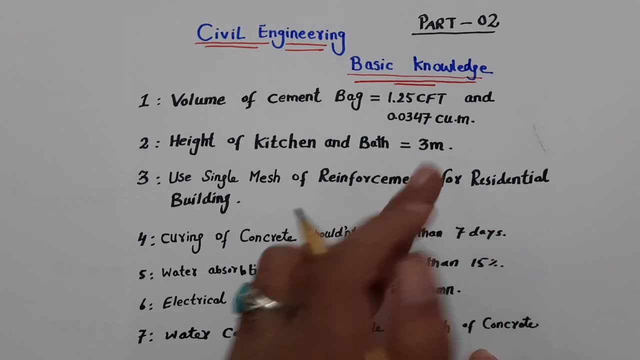 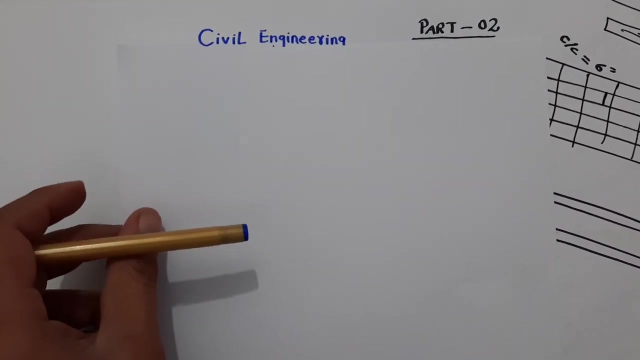 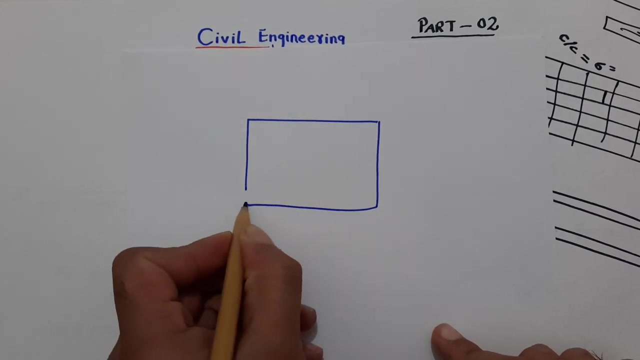 minimum three meters height of our height of roof. you can say should be minimum three meters. the third one is use single mesh of reinforcement for the residential building. single reinforcement mesh, single mesh. okay, how? as you can see the footing. so here and the footing, steel reinforcement. as you can see, these are the longitudinal bars. 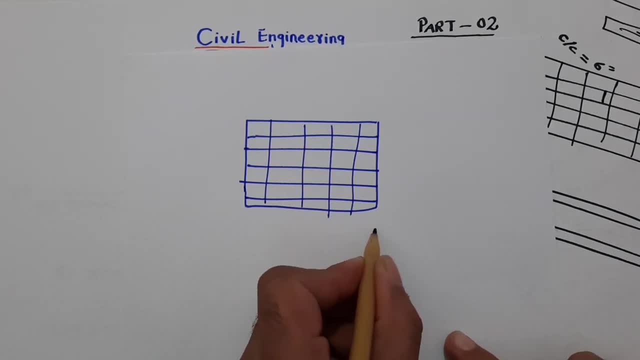 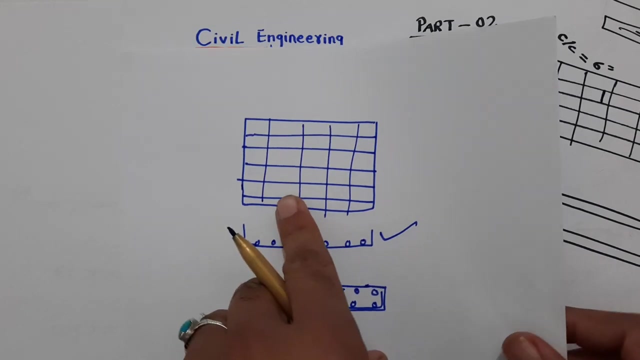 okay. so here in this cross-section you will see the. it should be singly reinforcement. okay, this one, but not this one. this is double reinforcement, guys. you can see here this is double reinforcement. so therefore, double reinforcement should be used for the mega projects are for commercial building, but singly reinforcement mesh should be used for the residential. 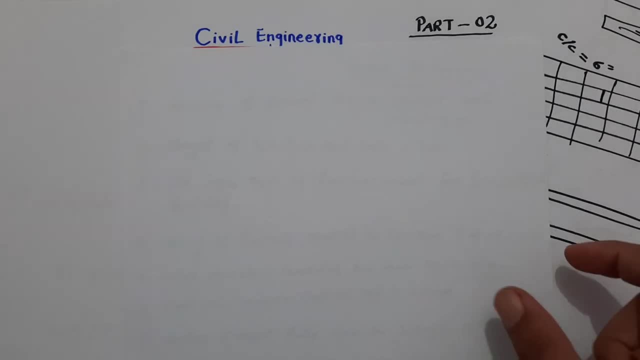 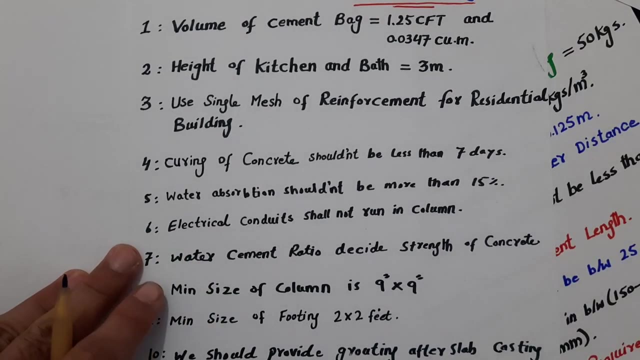 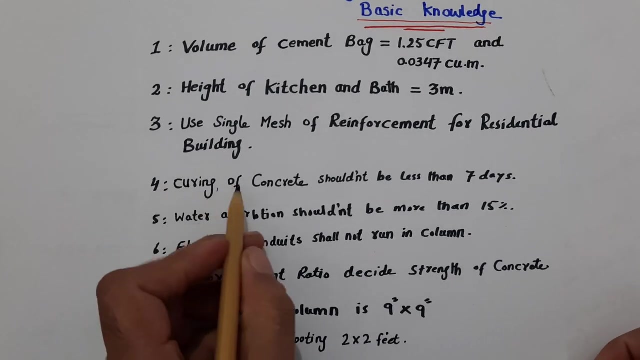 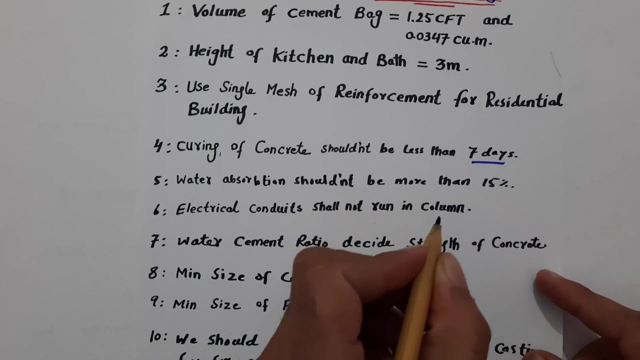 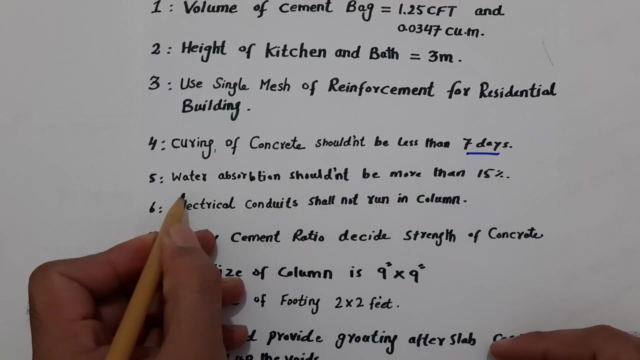 building. okay now, guys. the next one is: which is one second, guys? the fourth one is curing of concrete should not be less than seven days, so minimum the curing time should be seven days. okay, for any structure: beam, column, slip, okay, etc. minimum seven days. fifth one is water. 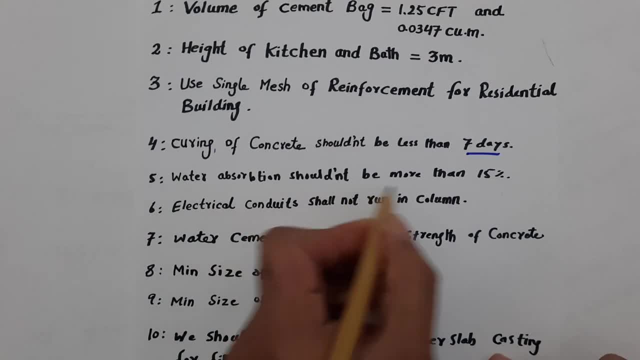 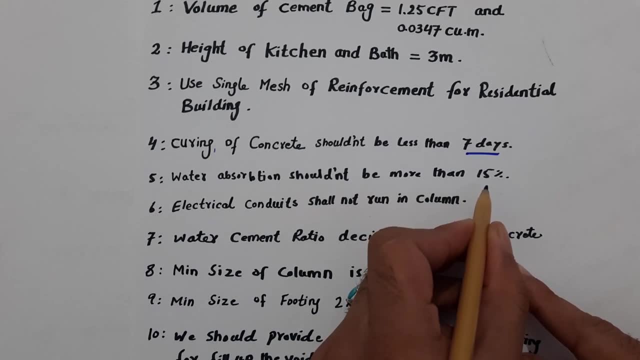 absorption should be. should not be more than seven days. okay, minimum seven days for any structure, beam column. Ergo, it should be more than seven days in Egypt, above one second on the base. it should be more than remained 15 per cent, especially for bricks, if any material absorbed more than 15 percent water. so 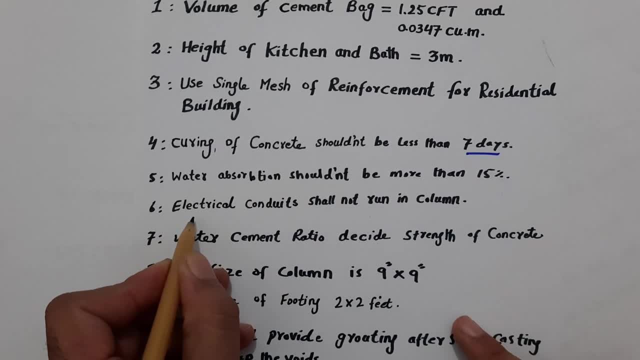 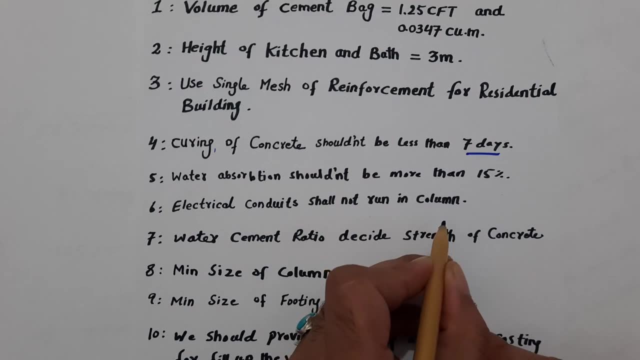 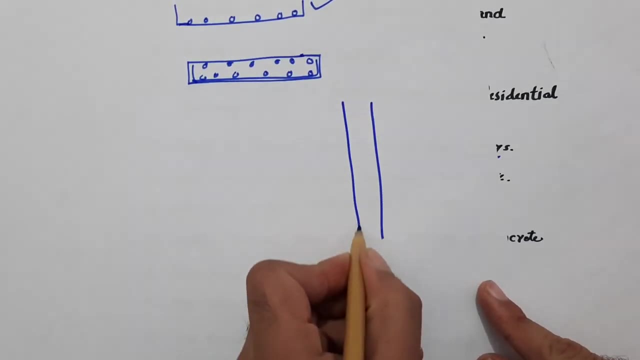 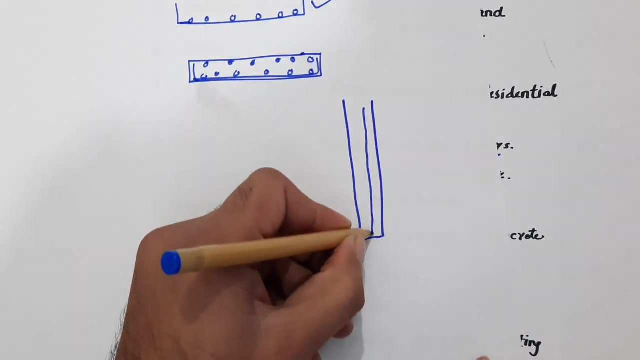 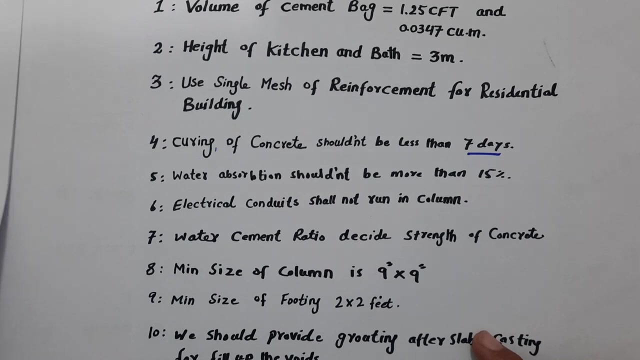 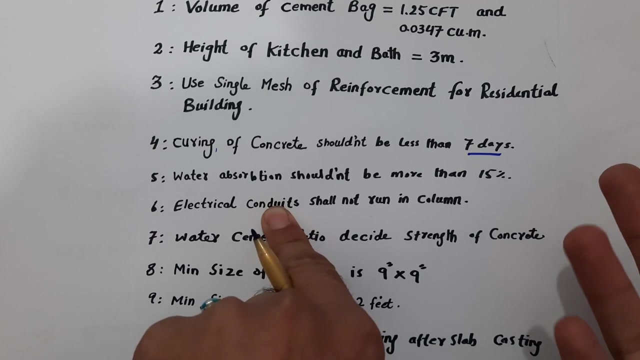 don't try, I don't use those materials and building construction. okay, not more than 15 percent. wars pubs: option the 6-10 is electrical conducts. our circuit shall not be run. This is column. So in most of the project I saw they are using PVC pipes for the rainy waters inside the column. Okay. So, guys, this is wrong. Don't run any electrical circuits or conducts or PVC pipes for the rainy water or for the sanitary. Okay. 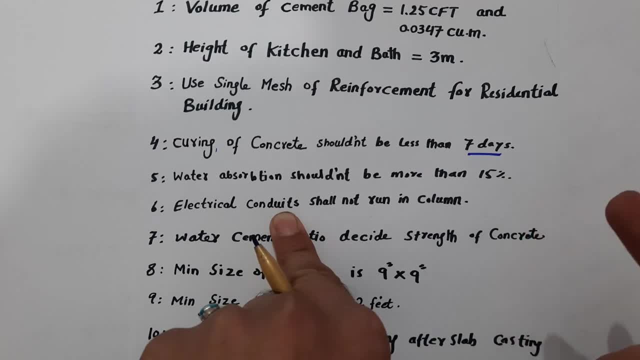 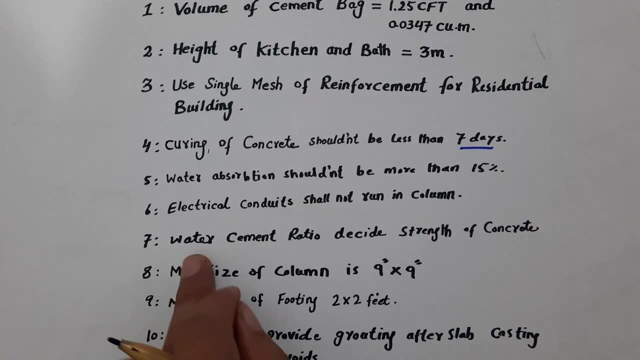 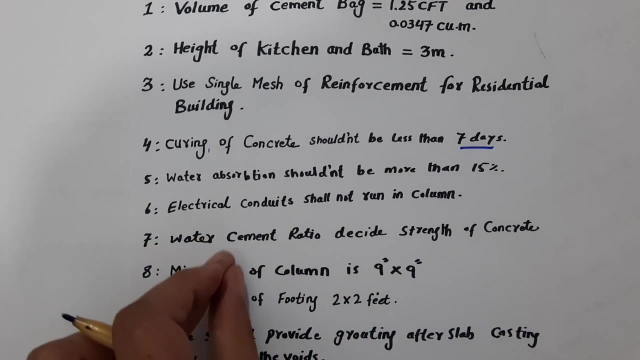 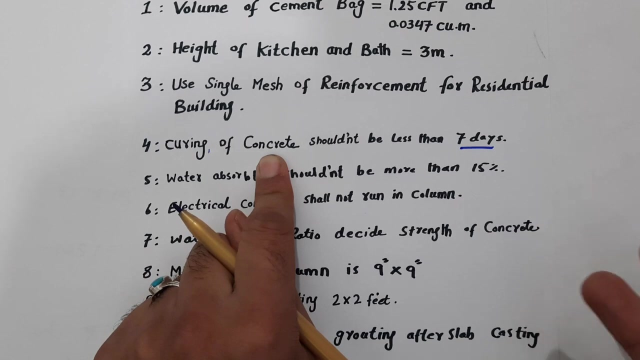 So electrical conducts or other rainy water pipes should not be run in a column. Okay, The seventh one is, guys, water cement ratio decides strength of concrete. Water cement ratio decides strength of concrete. If you increase the water cement ratio so it will increase the workability. So when you have more workability so the concrete is not strong. 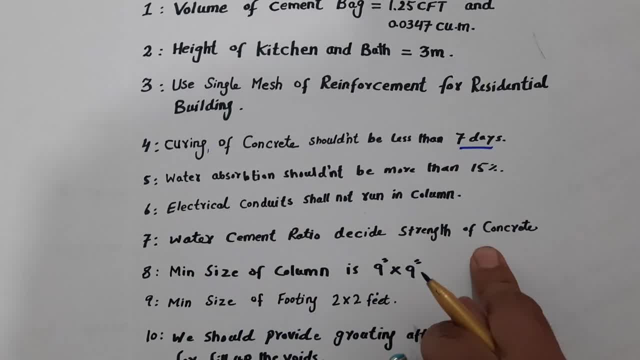 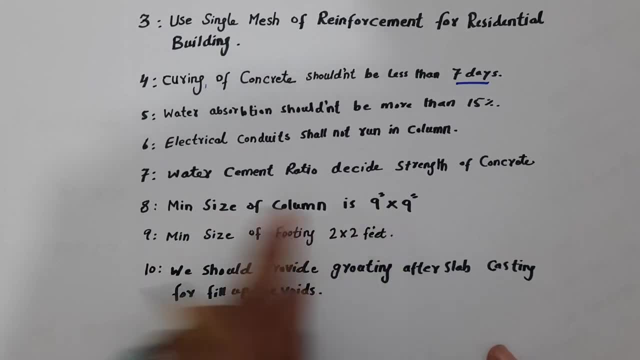 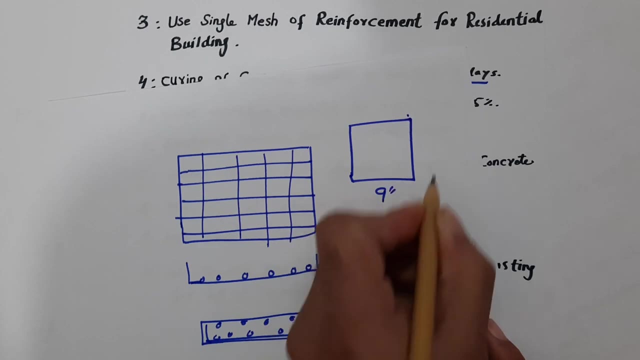 Okay, So water cement ratio decides the strength of concrete. This is the technical term. Okay, The next one is: guys, minimum size of the column is 9 by 9 inches. As you can see, this is column, So the column size should not be less than 9 by 9 inches. Okay, Especially for commercial building. Okay, 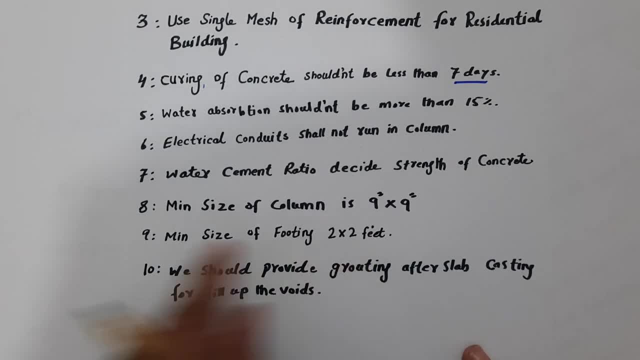 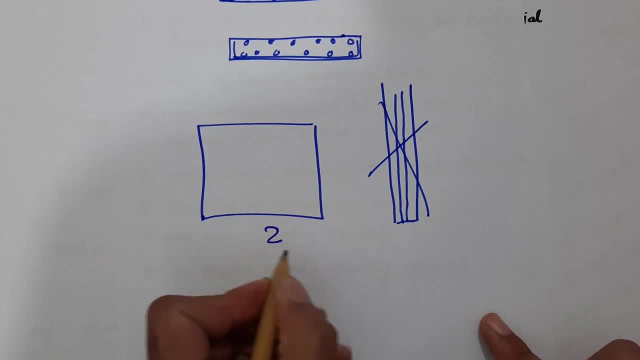 Ninth one is minimum. size of the footing should not be less than 2 by 2 feet. As you can see, size of the footing should not be less than 2 by 2 feet. Okay, This is the minimum size of the footing: 2 by 2 feet. This is minimum, as you can see inside column Okay.